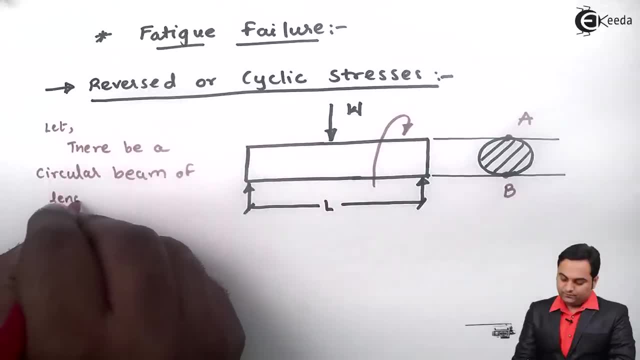 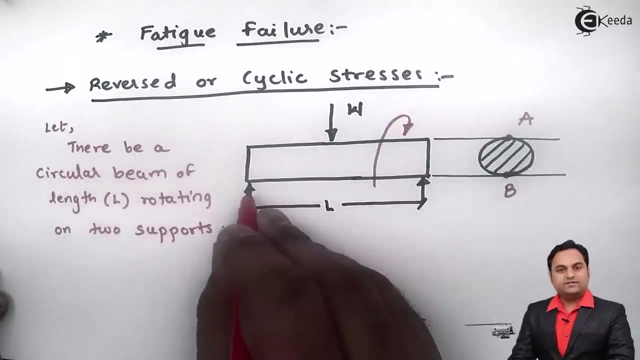 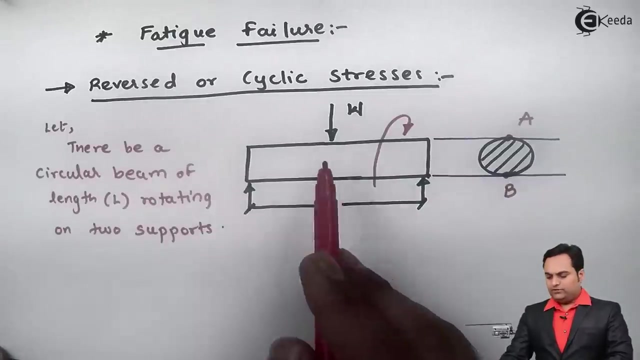 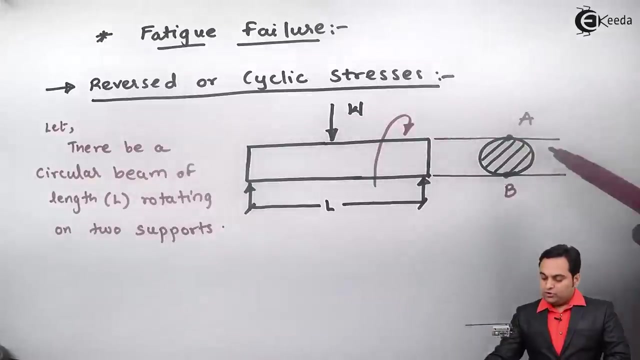 at this place. 11.好了 earned rotating on two supports. so here in the diagram, as i can see, the beam is supported at two ends and we are considering that it is rotating now because of this load, since the beam is rotating and at the same time there is load acting over this. so what happens? supposed at first instant? 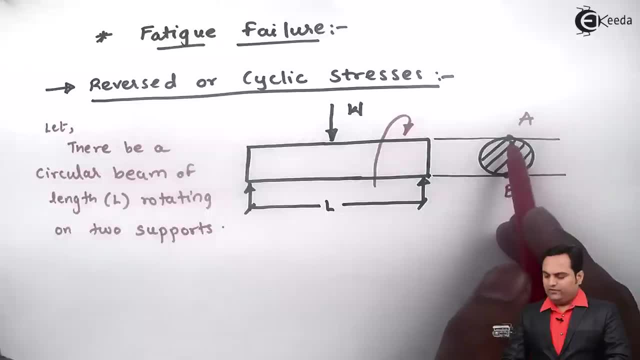 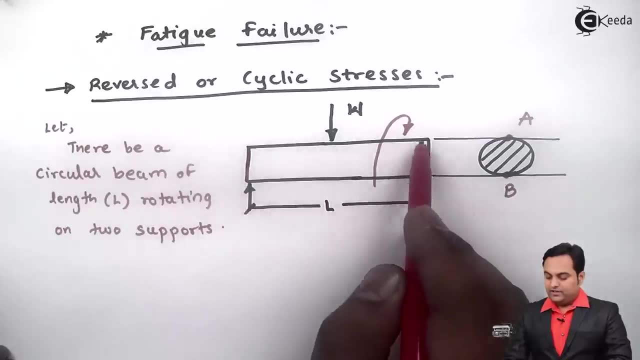 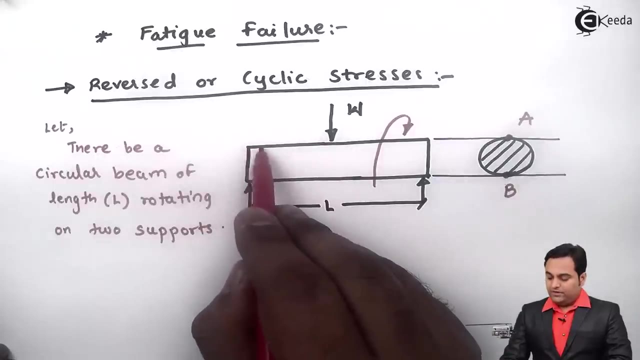 the load is acting at point one, or we can say point number a. now, if a is at the top, i can say this top layer is a, bottom layer is b. then, when load is acting, the top layer of the beam will be compressed because of the load, whereas the bottom layer, it will be in tension, it will be elongated. 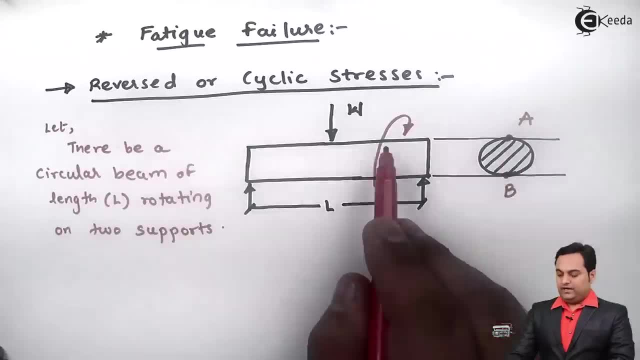 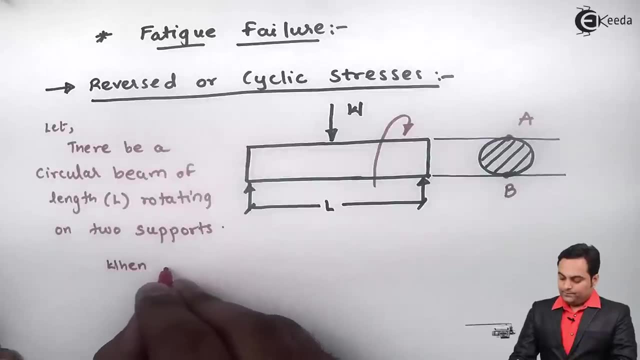 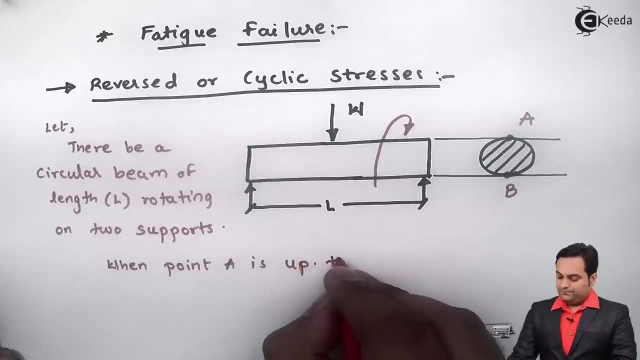 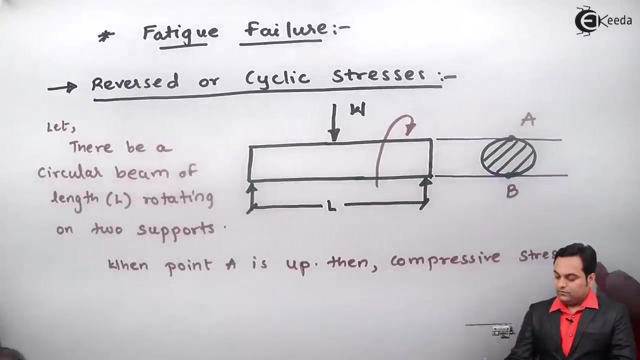 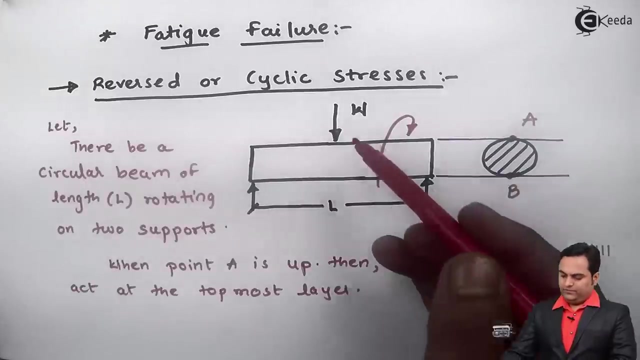 that is, if point number a is at the top. so i can say that when point a is up, then compressive stress will act at the top most layer. so as i can say that when this load is acting at the top most layer, there will be compressive stress, 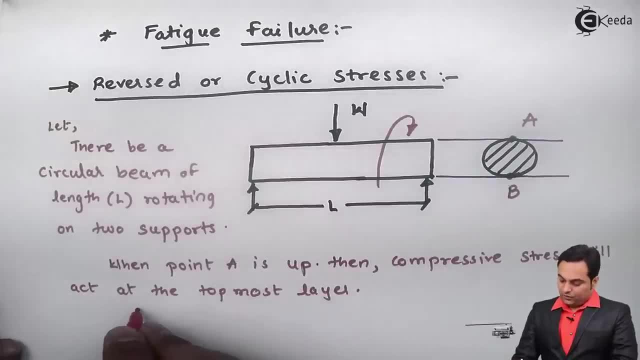 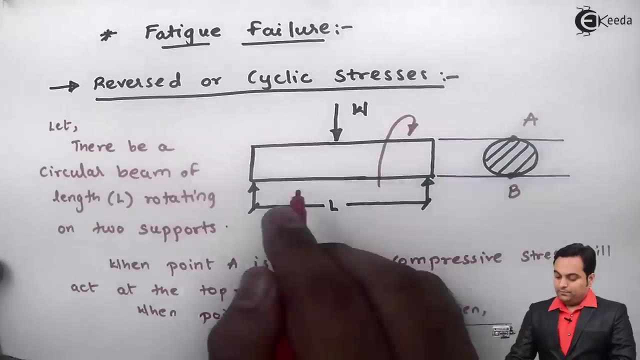 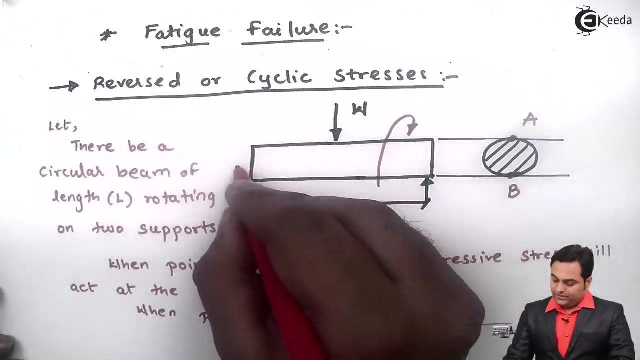 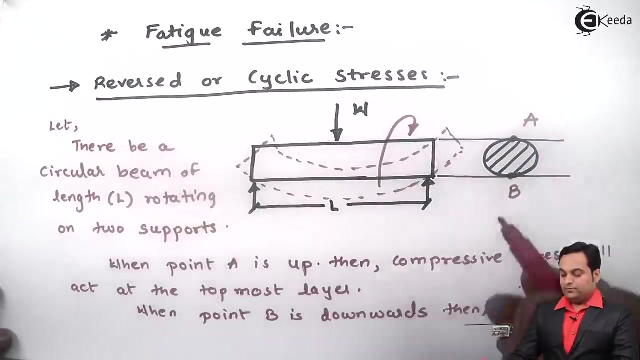 or i can say: when point b is downwards, then b would be subjected to tension, because we know. so, as i can see, the upper layer is subject to compression and the bottom layer, that is at point b, since it is downwards, then tensile stress will act at the bottom, which is located at the bottom. 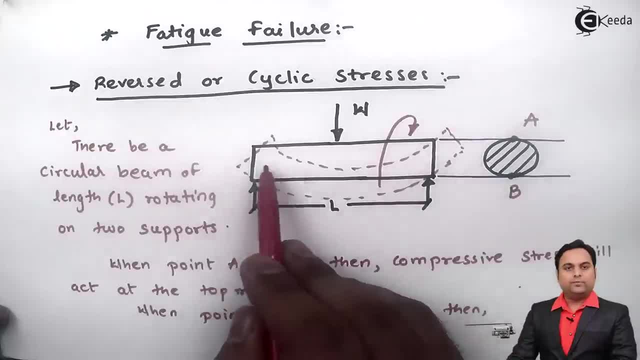 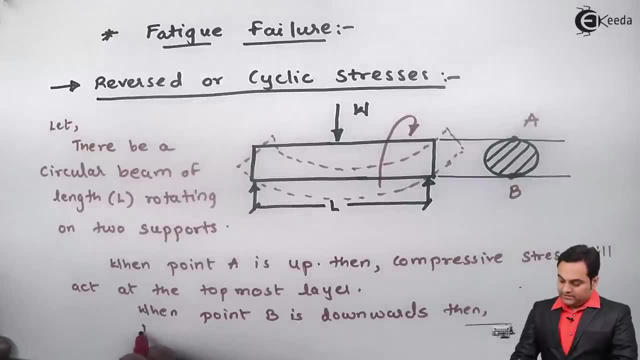 so the third way is that the resistance of the beam is not attenuated to the top layer. we have simply supported beam here. and the bending pattern of a simply supported beam- here i have simply supported beam- it will bend in this way. here i am drawing the diagram and indicating it will be bending in such a way. 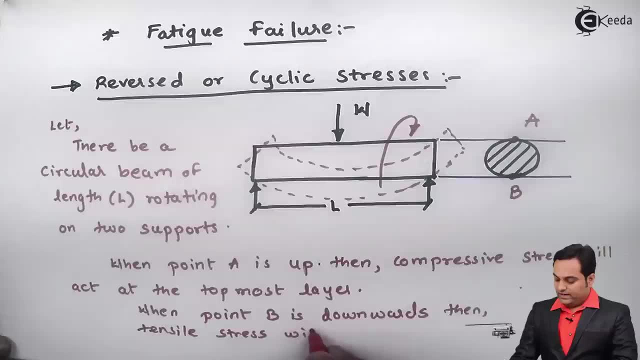 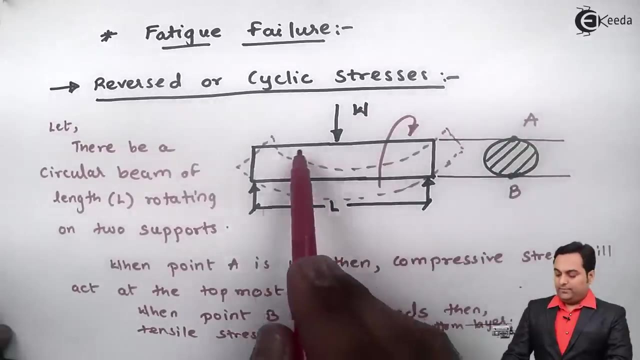 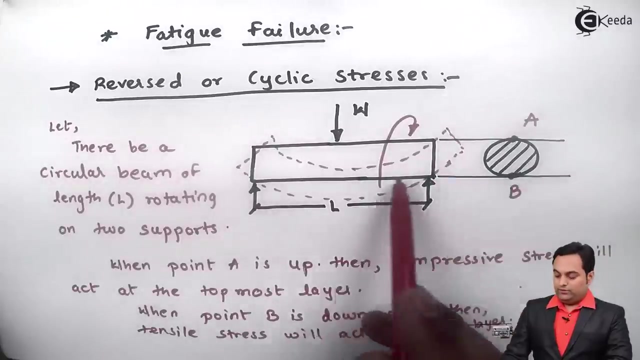 will act at bottom layer. so here it is clear that when the load is acting and point A is up, A, which is the up top most layer, it will be subjected to compressive stress and the bottom most layer, that is layer B, it would be subjected to tensile stress. that is when 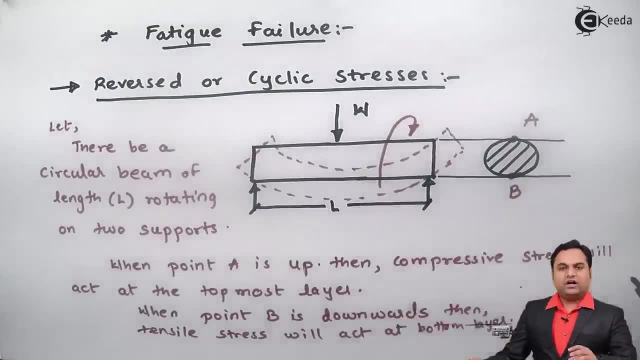 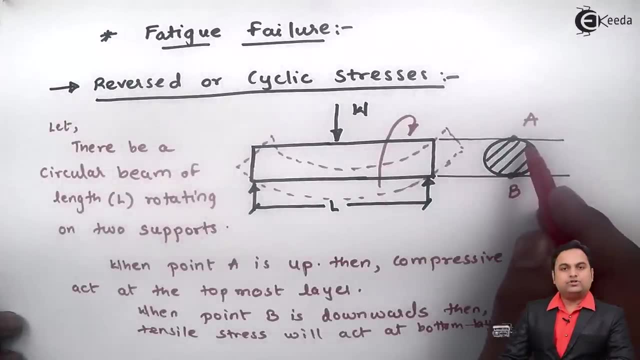 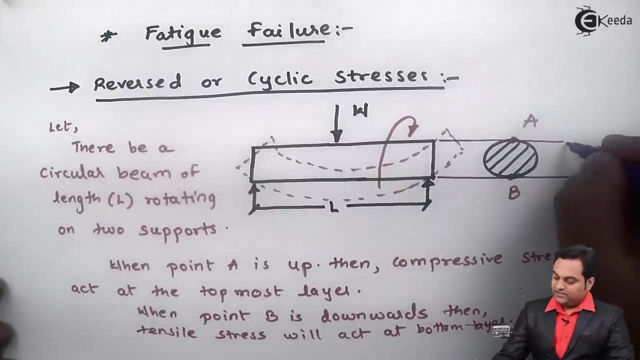 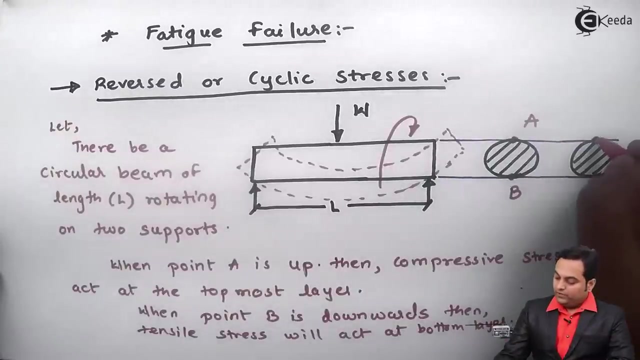 point A is up. Now take an example that this shaft is rotating. so in next turn what happens? instead of A point, number B goes up, that is, B becomes the upper layer. so now, if I say that for the second case, then the shaft will rotate, then point B will reach up, whereas point A will be at the bottom. 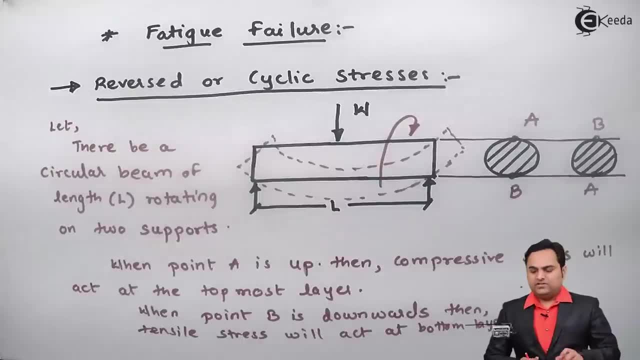 So now the action is reversed. previously A was subjected to compression and B was in tension. now, since point B has reached up, because the shaft is continuously rotating, So each of the points, they would be shifted. So when B reaches the top, most layer, now, B would be subjected to compression and A would 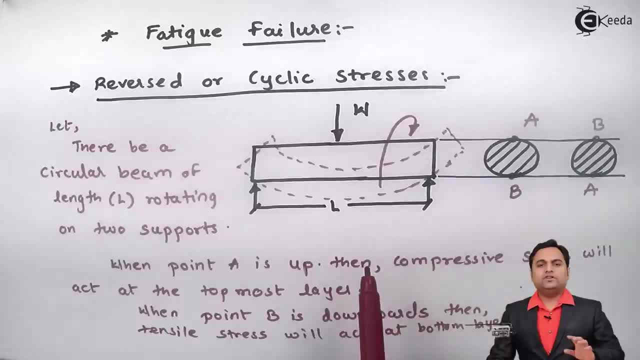 be subjected to tension. So this is called as reversed or cyclic stresses, where a particular member, or we can say a particular point, is subjected to two kinds of stresses in the same cycle. So here I can say that, since I have written for point A and B, 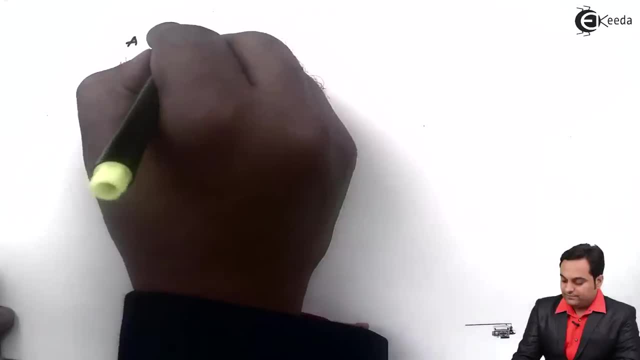 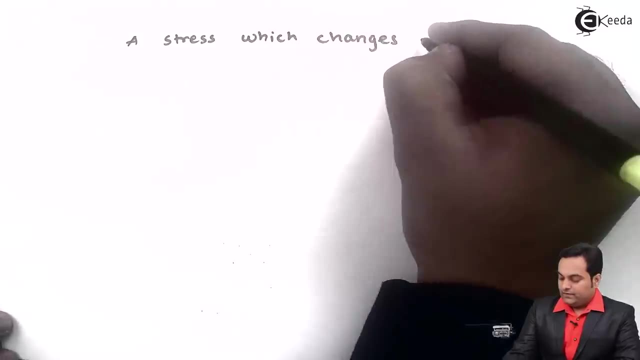 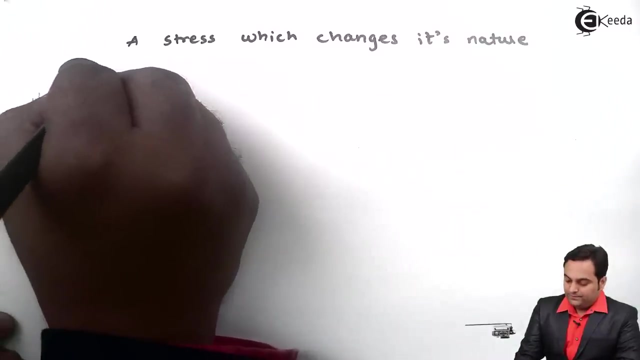 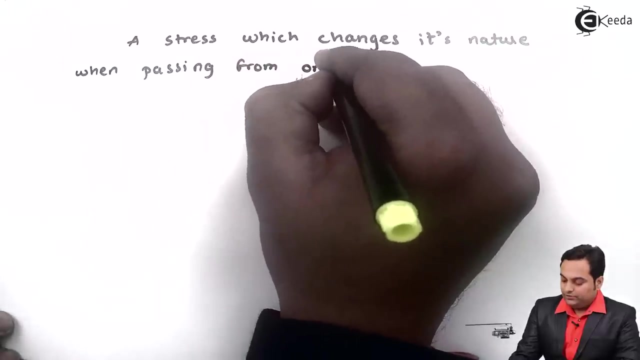 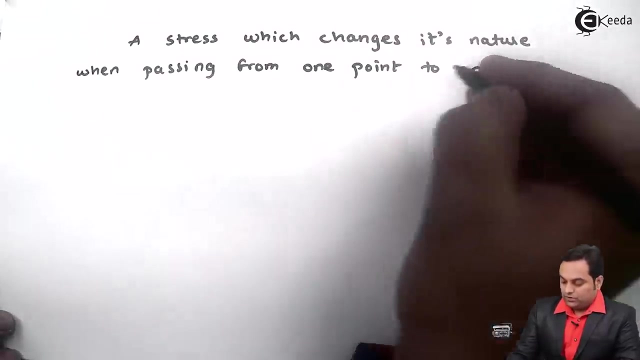 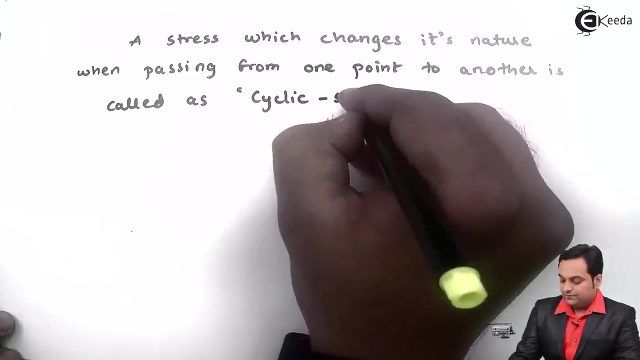 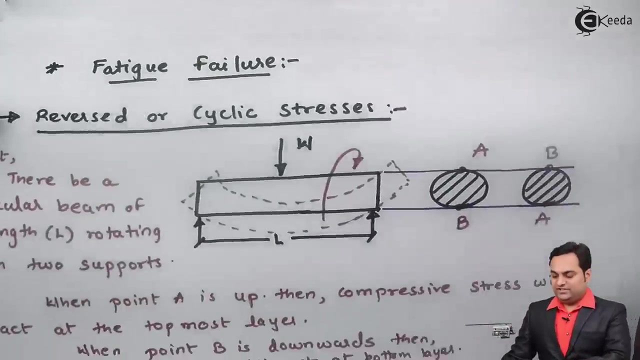 I will say that a stress which changes its nature when passing from one point to another point is called as cyclic stress. So here I have written a stress which is changing its nature. Nature means at first point A was subjected to compression when the shaft has rotated. 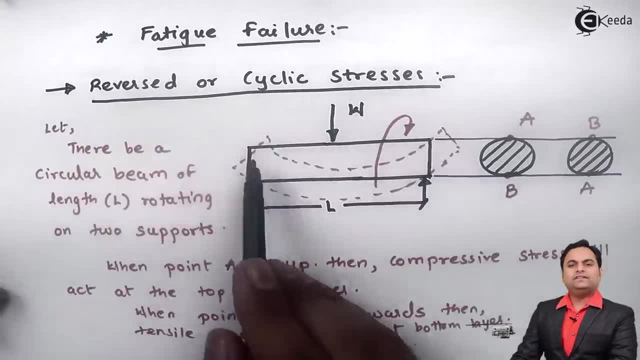 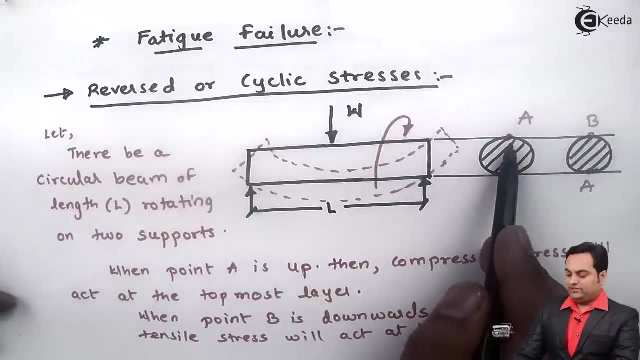 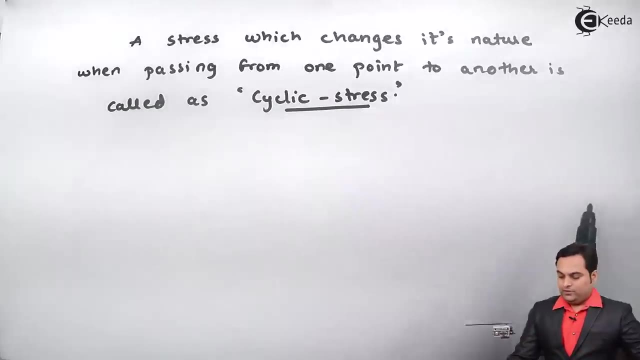 now point A is subjected to tension. So the nature has changed top layer. first it was at point A, Then the top layer is at point B. So at first A was subjected to compression, next A was subjected to tension. So the nature of stress has changed. 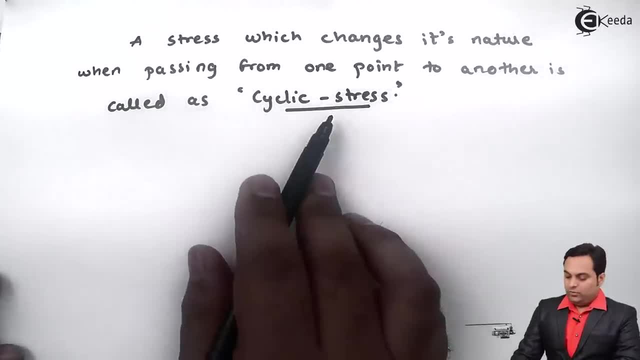 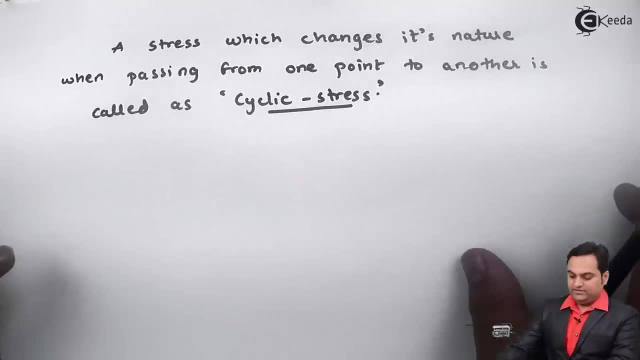 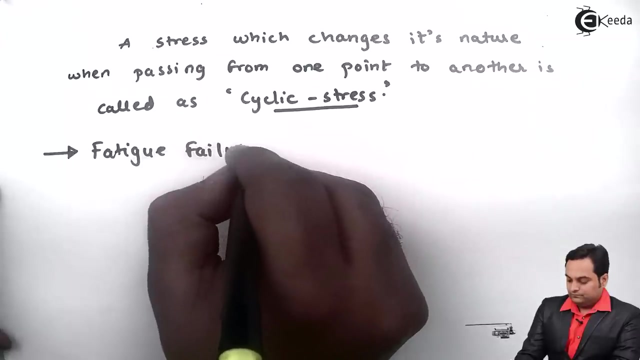 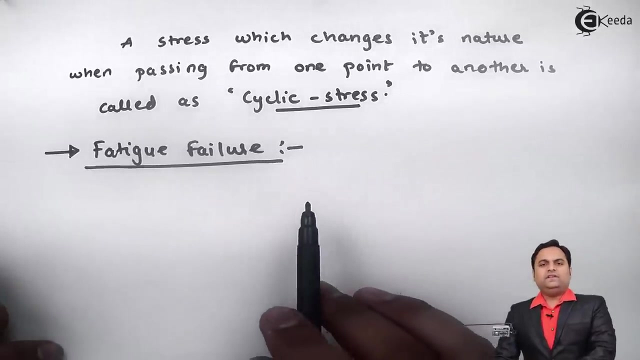 So from one point to another it is called as cyclic stress. Now, once we understood what is cyclic stress, then we can easily go for fatigue failure. So here I will write down: after cyclic stress, fatigue failure. Now in fatigue failure, as we have seen in cyclic stress, the stress changes its nature. similarly in fatigue failure, the load which is acting, it will change its direction and it will change its value. that is, the same machine member will be subjected to different values of load and in different directions. so it is somewhat similar to reversed or cyclic stress. So fatigue failure, it is a kind of failure in which the load changes its magnitude and 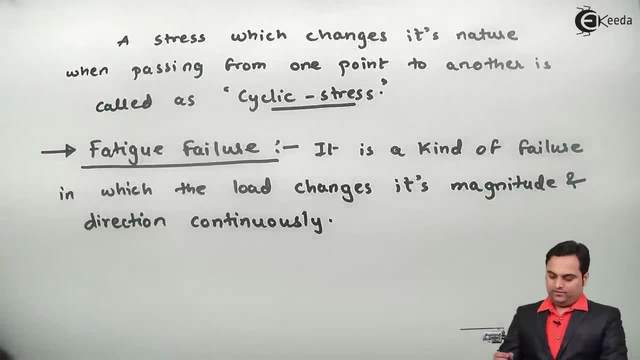 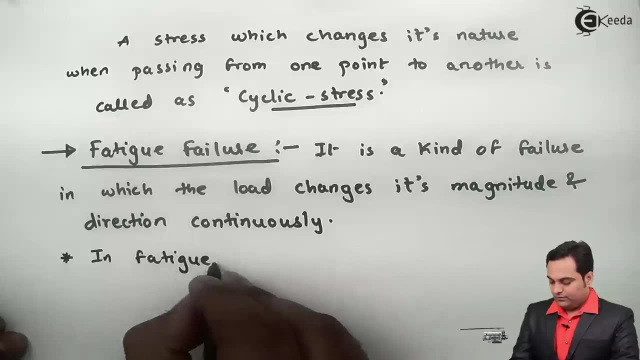 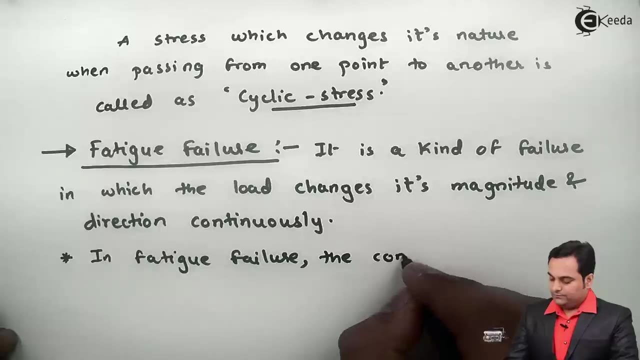 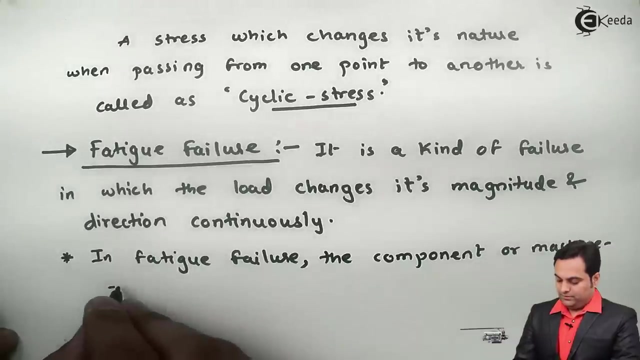 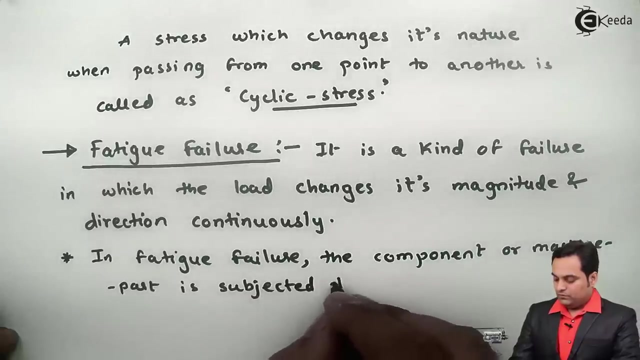 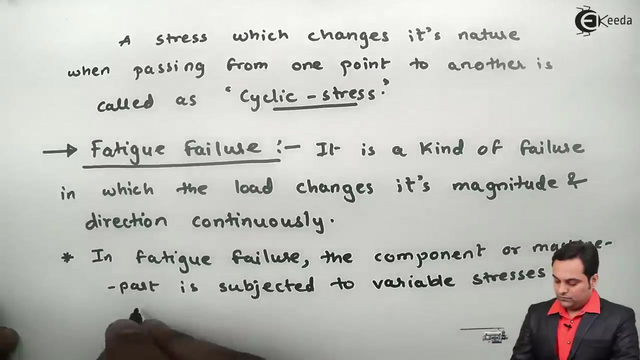 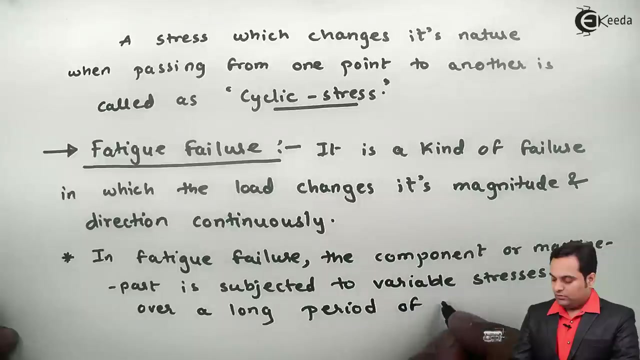 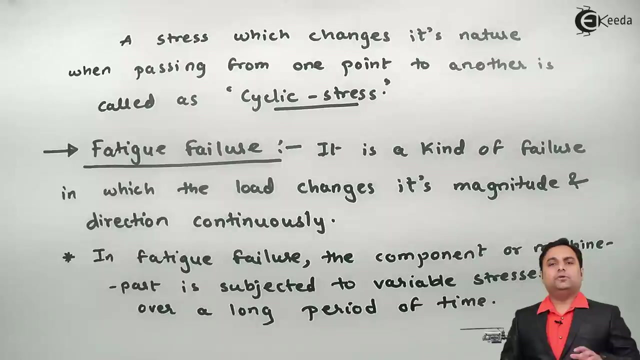 direction continuously. Next, Next, Next. in fatigue failure, the component or machine part is subjected to variability, Variable stresses over a long period of time, as I have written here. in fatigue failure, the component or a product or a machine part- we have it- is subjected to variable stresses. 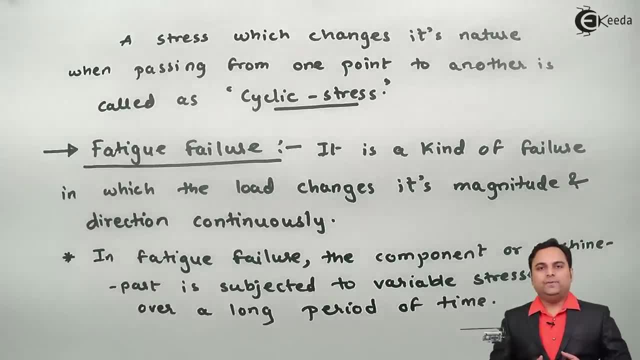 means the stresses. they continuously go on changing their value and it is subjected to these stresses for a prolonged period, for a continuous period or we can say over a long time. So fatigue failure is mostly seen in those components or products which are used over time, that is, which are used for number of years and they are subjected to variable stresses. 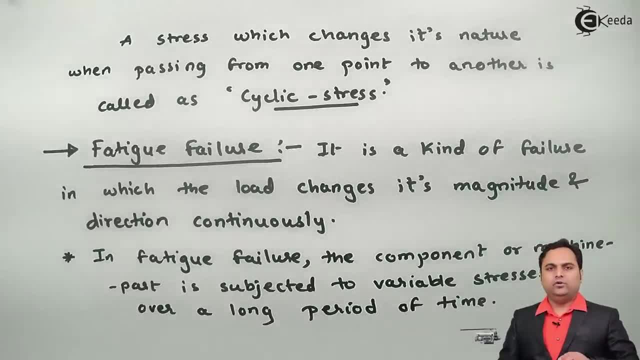 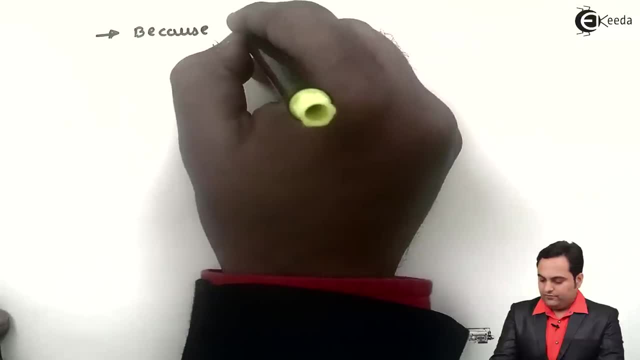 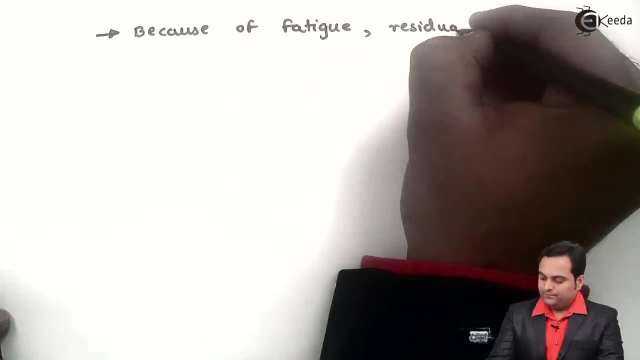 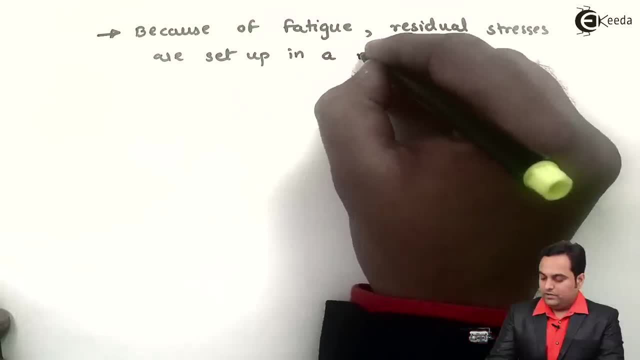 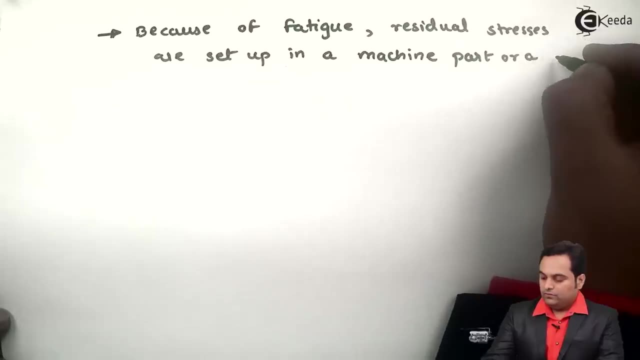 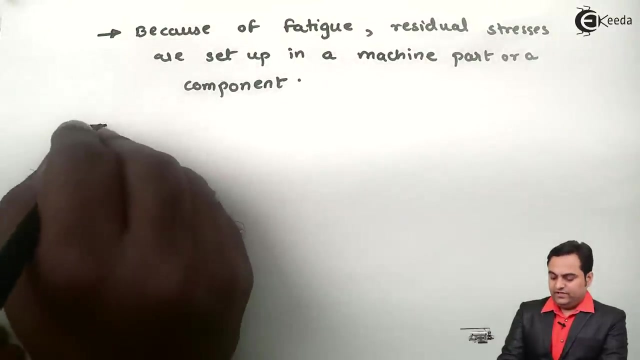 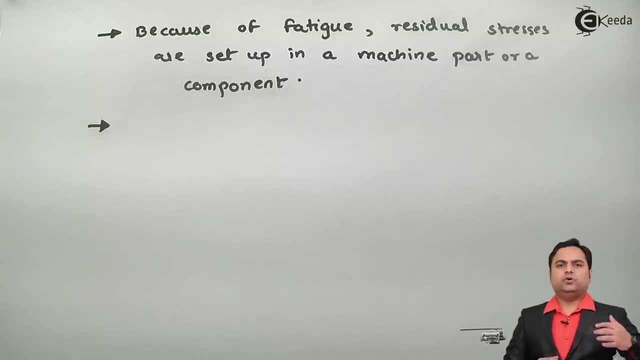 various types of stresses, various values of stresses, over long period of time, that is, for number of years. then what happens? some stresses which are residual, they get stored in that material and over time, if certain value or some some value of load is acting on that machine part, it may develop inside cracks and that cracks once it reaches inside. 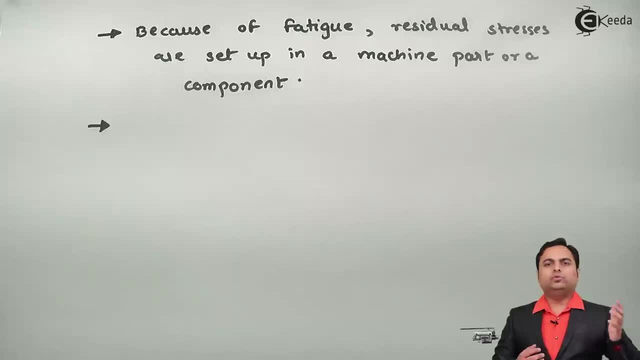 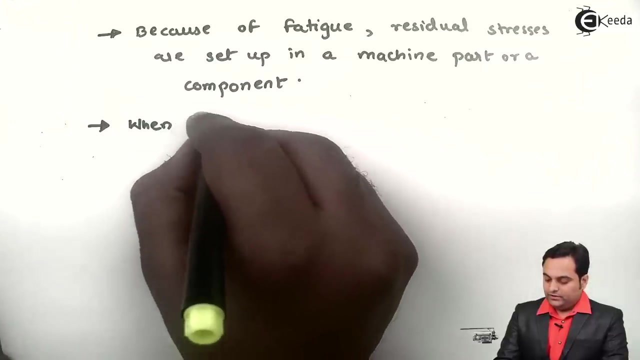 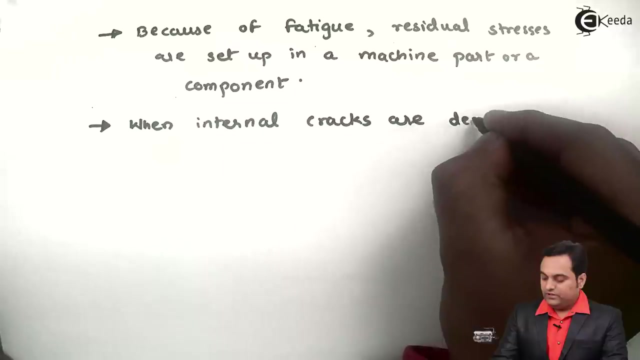 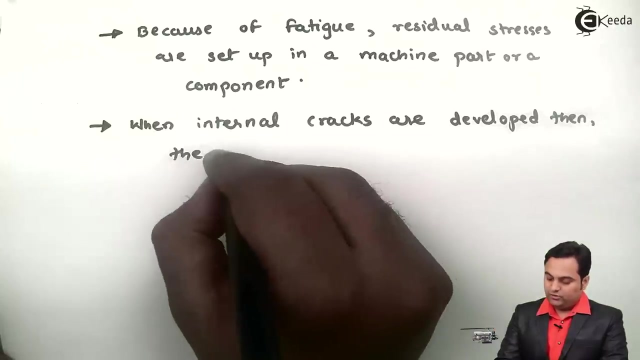 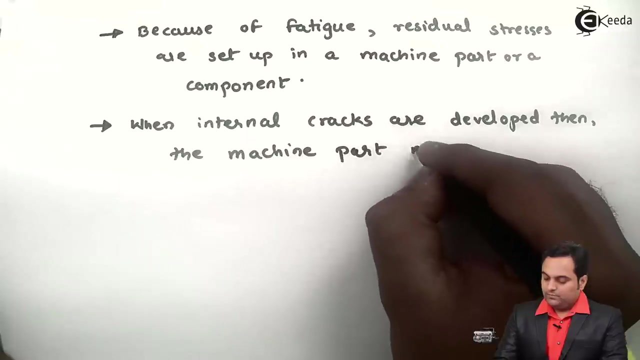 the surface, then it will be propagating, it will move towards the surface from inside to outside and finally the object would be breaking. so here i can write down that when internal cracks are developed, then then the object or a product or we can say machine part, may fail anytime. that is even a small. 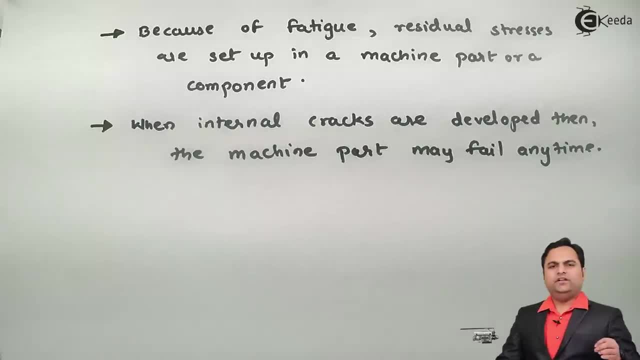 value of load is necessary or a very small value of load can break that machine part because through the number of years, for a long period, it was subjected to number of stresses which were changing their direction As well as their value. because of that, fatigue developed inside the material. and when a small 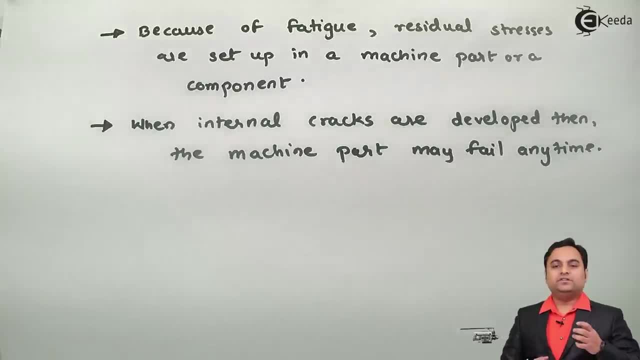 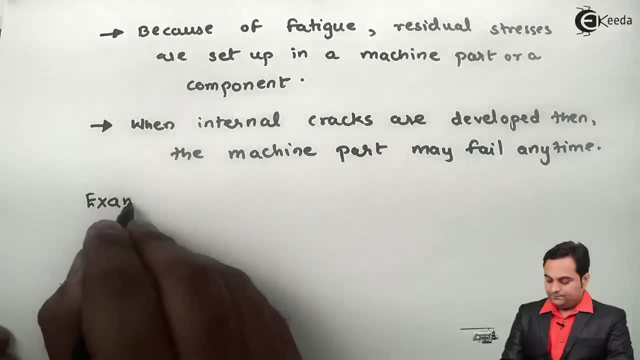 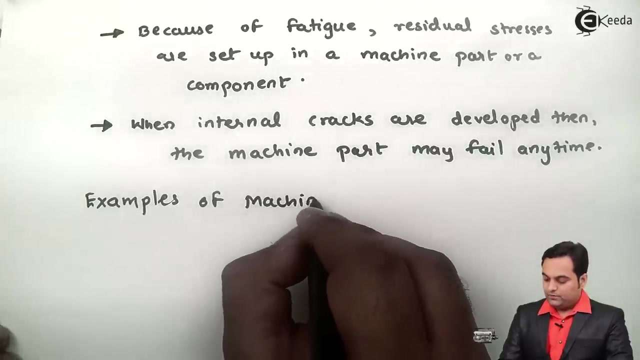 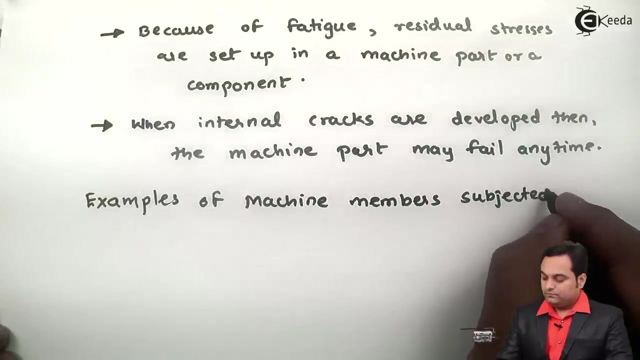 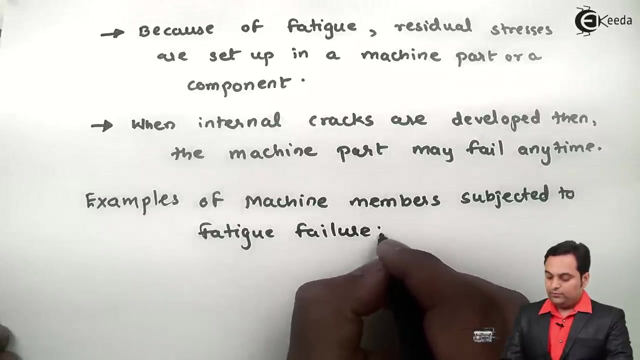 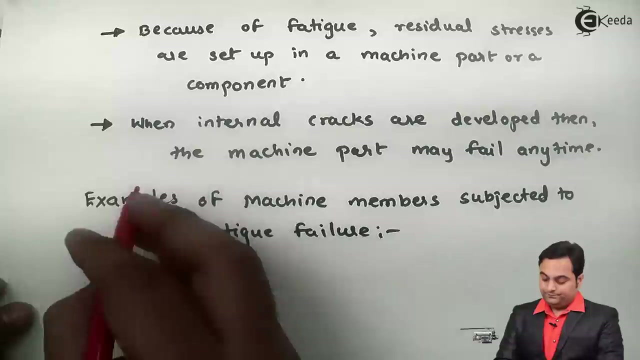 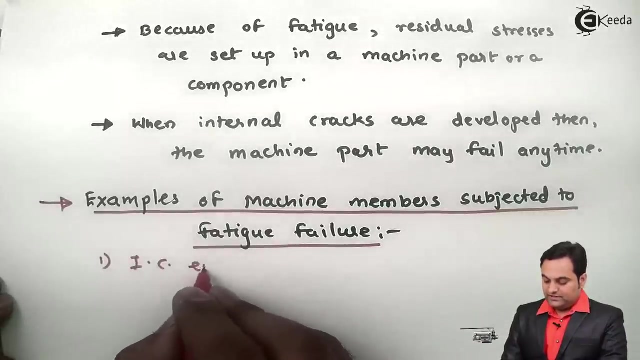 load reaches that object, it results in internal cracks and then the failure of the material starts. so I can give the examples of machine members Subjected to the load to fatigue failure. see fatigue failure is more prominent in those machines which are used over a number of periods. so I can give the examples, like we can say IC engines, that